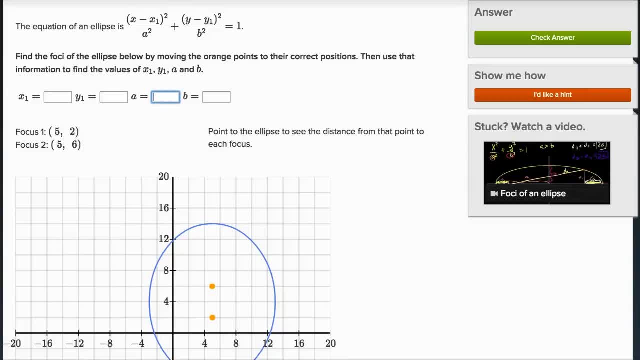 I thought it would be interesting to get a little bit more intuition on ellipses and their foci, or foci. Sometimes I like to call them focuses, but the correct word is foci or foci, but either pronunciation is apparently okay. So let's work with this. This is an interactive exercise 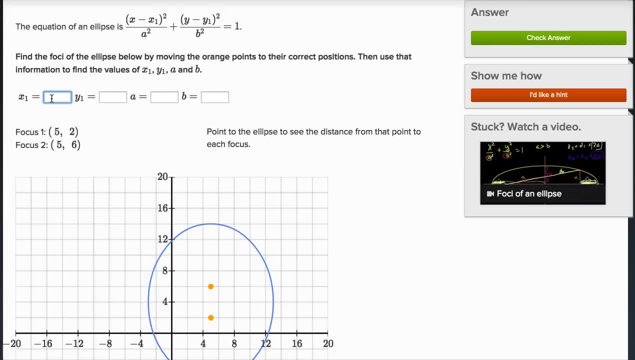 on Khan Academy's you see over here. So let's see if we can work through this together and learn a little bit more about ellipses. 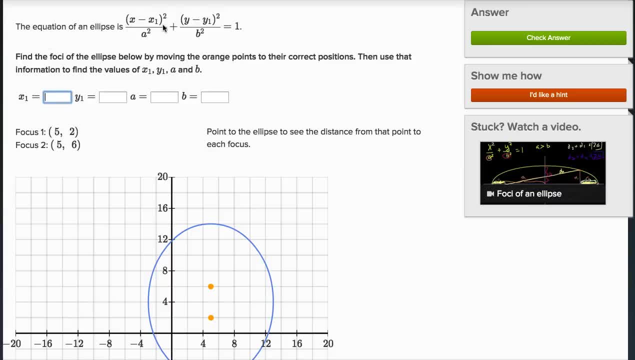 So they tell us the equation of an ellipse is x minus x one squared over a squared plus y minus one squared over b squared equals one. 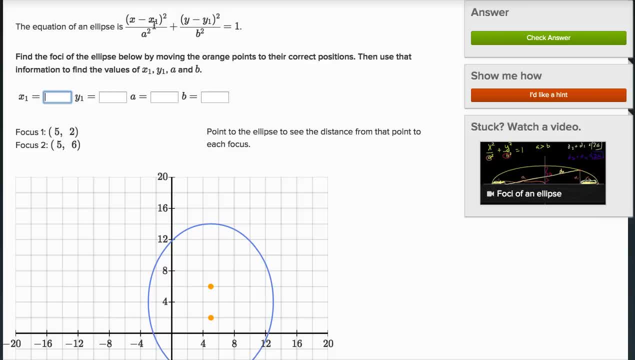 And this is true. This is the equation of an ellipse. This would be an ellipse that is centered 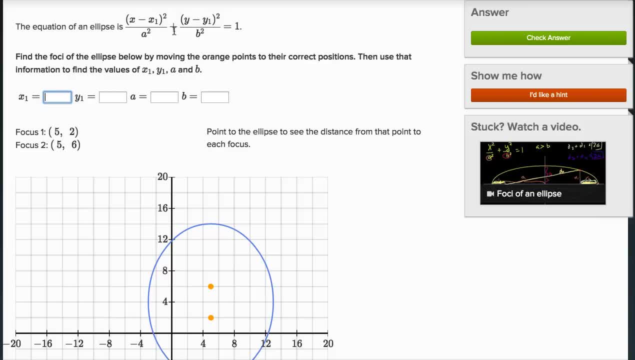 at x equals x one, y equals y one. The major radius would be a. The minor radius would be b. 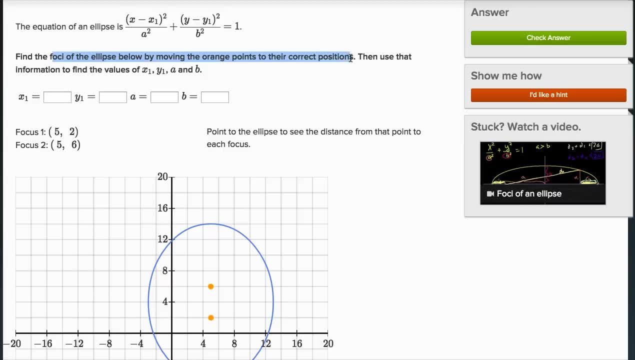 So then they say find the foci of the ellipse below by moving the orange points to their correct positions. 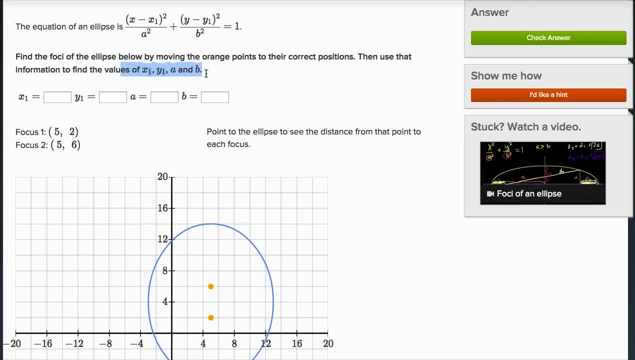 Then use that information to find the values of x one, y one, a and b. 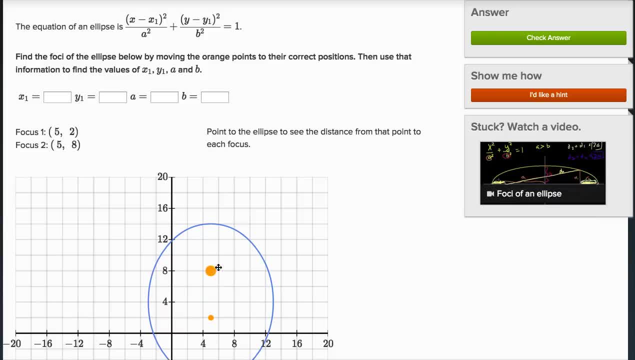 So they want us to move these to their correct position. The correct position is where the sum of the distance, so if we move it to the correct position, the sum of the length of that red line and the length of that green line should be constant. 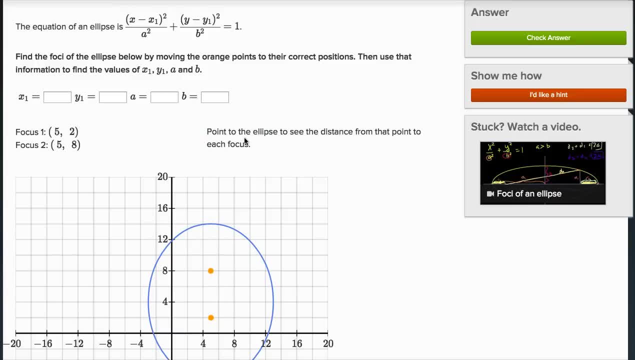 Now you can see they're clearly not in the correct position right over here because up here when I was moving it around, you see that, look, the distance to foci one from this point on the ellipse is 11.7. That's the green line. The distance to foci two is six. You add them together, 17.8. But when you move it around, that changes. 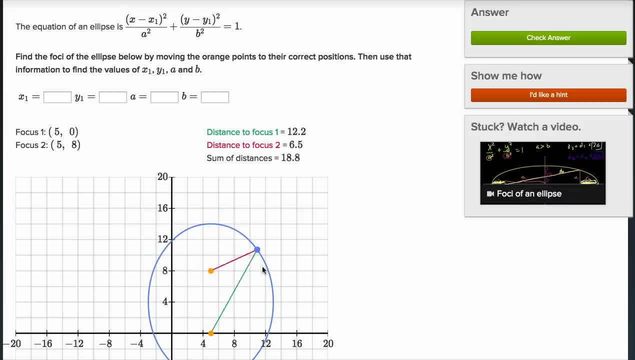 And so we would have to find a different, we could just keep trying different foci until that sum of these, the red length and the green length is constant. 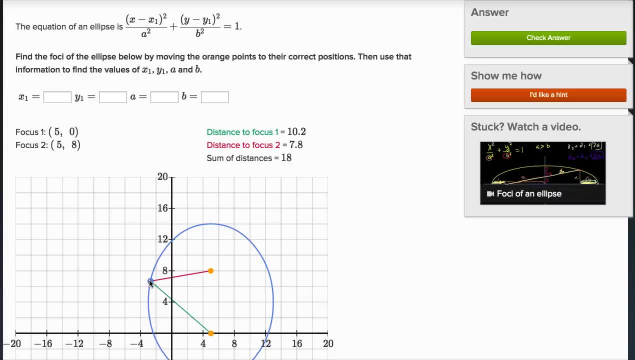 Now in my mind, that is a hard way to do it. An easier way to do it would be, well, let's figure out the center of the ellipse first, which we could do just literally by inspecting this drawing, and then figure out what the length of the major radius and the minor radius is, and then use that information to find the foci. 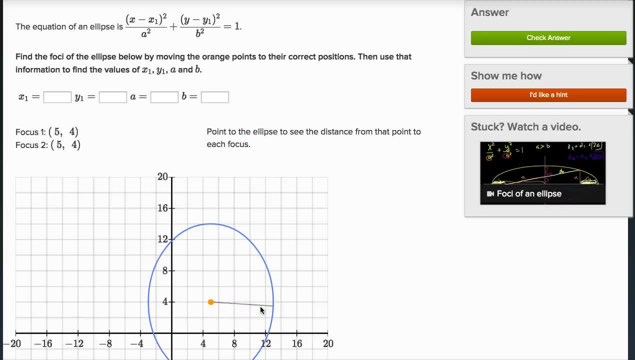 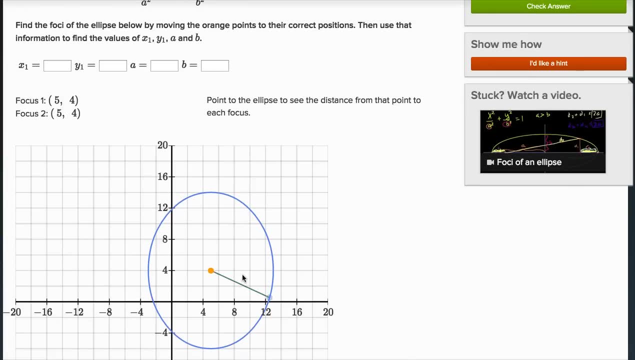 So let's see if I can put these dots, let me put them first at the center. All right, so let's see. So that center, and let me, that looks pretty good. That looks like the center, and I can even confirm. So in the y direction, that is, if I'm at the top of the ellipse, I am 10 from that center, and if I'm at the bottom of the ellipse, I am 10 from that center. 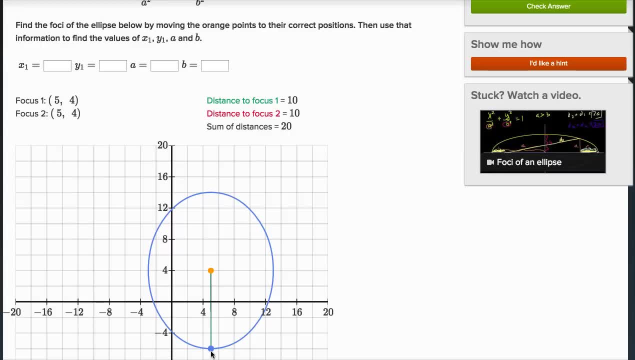 And so that does look like the center, and it also tells us, it tells us that the, 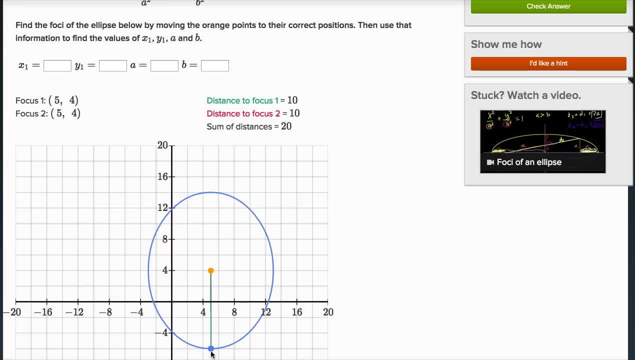 that the major radius is 10, and it's along the y axis. 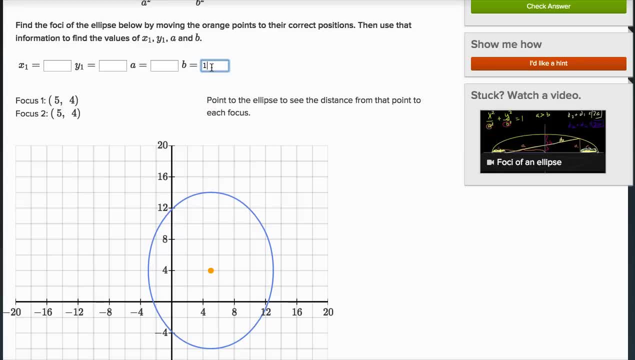 So the major radius is 10, and it's along the y axis. 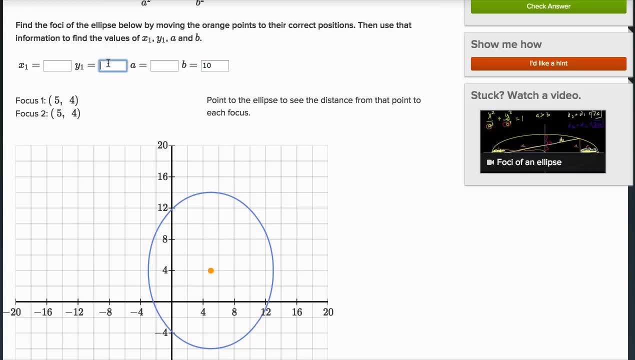 And we also know the y coordinate of the center, it's y is equal to four. Y is equal to four. 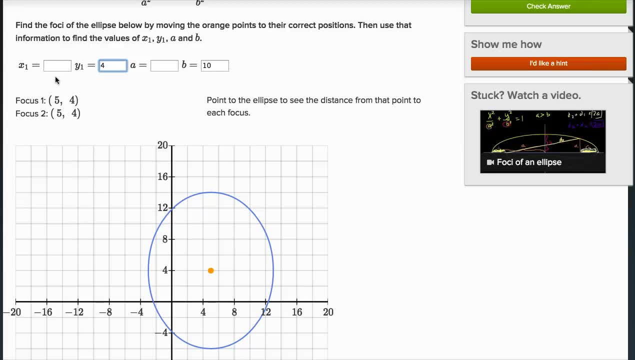 And then the x coordinate of the center is x equals five. 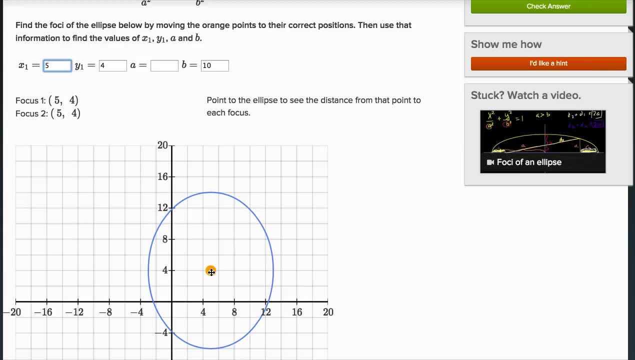 So once again, where I put this orange dot, that is the center of the ellipse, it's at x equals five, y equals four, and that's why I put x equals five, or x one equals five, y one equals four. 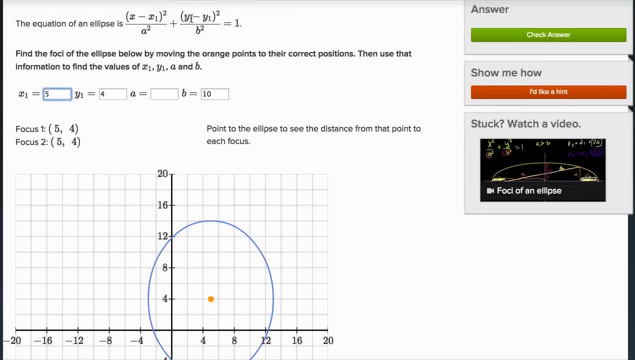 And you see from the equation of ellipse, that's what defines the center of the ellipse. And then a is going to be, a, we can see from here, this is the radius in the x direction. 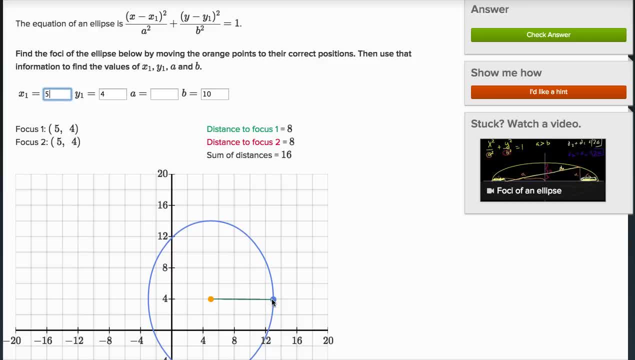 I guess you want to think about it. And that's going to be the minor radius, it's the shorter radius. And you see that has length eight. We're going from x equals five to x equals 13. Or x equals, or x equals negative three to x equals five. So it has length eight. So this thing right over here, a, is going to be eight. So this is eight. 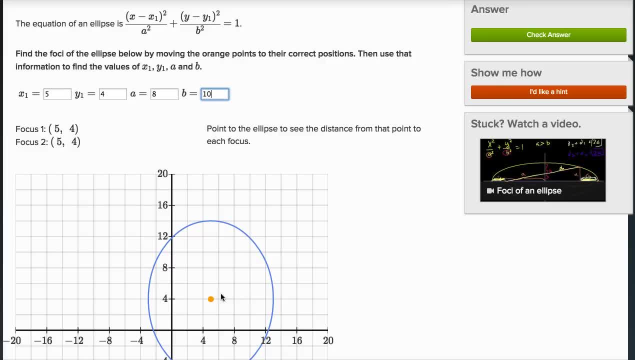 And we already said, the major radius is going to be in the vertical direction, and it is of length 10. So just like that, we figured out, we could write the equation down. I don't have my pen out, but you could just say, the equation of this ellipse is going to be x minus five squared over eight squared, plus y minus four squared over 10 squared equals one. 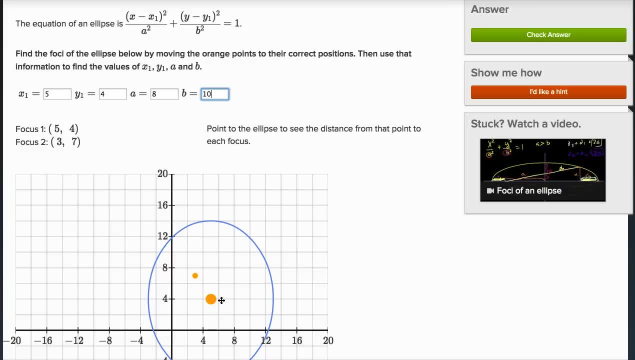 But now let's actually figure out where we need to put these foci, and then figure out that, hey look, if we put them in the right place, the sum of the red and green lines is going to be a constant. And clearly where they are right now, it's not a constant. You see that sum of the distances is at 20.6, and then it goes to 20 point, it's clearly not constant. 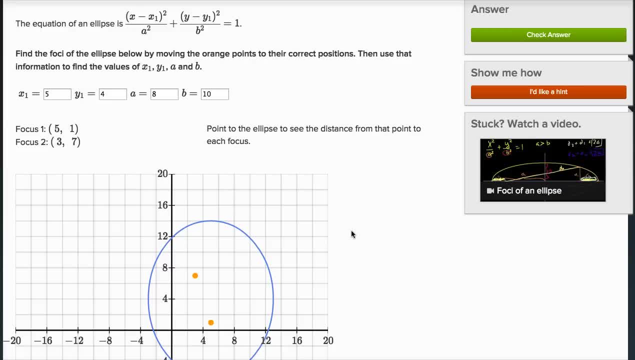 So let's see if we can do it. And one way to do it is just to remember, well there's a formula, and we talk about it, we explore the intuition behind it, in a few minutes. 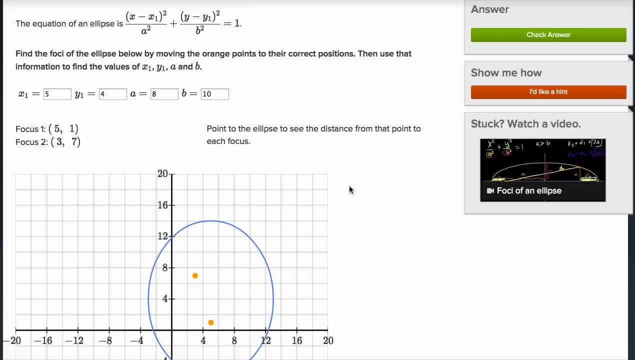 This is from a previous video. But the formula for the foci ellipse is, you find the difference between the larger of these two values and the smaller of these two values. 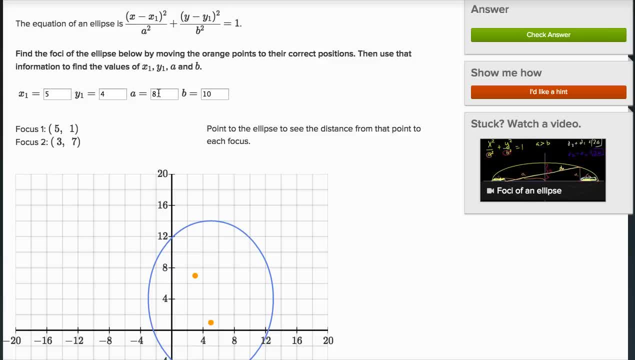 So in this case, you would find the difference between 10 squared and eight squared. Well that's going to be 100 minus 64, which is 36, and then you take the square root of that. 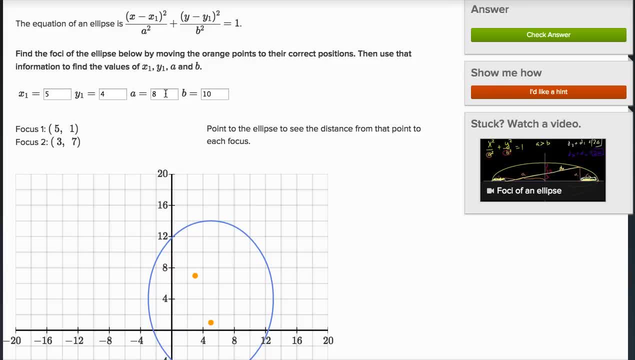 So it's going to be equal to six. So the focal length is going to be equal to six. So if we go back to the center, if you go back to the center, 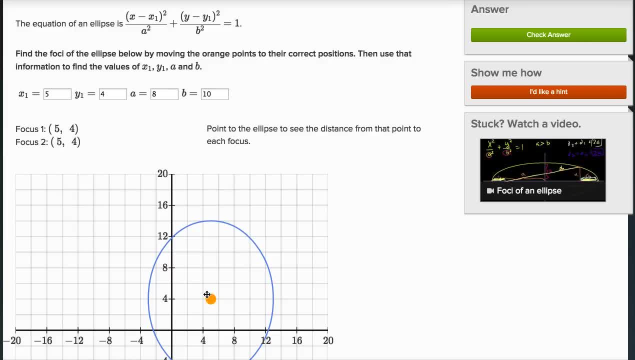 if we figure out our focal length is six, and remember all I did is I took the larger of these, I squared it, and from that I subtracted the other one squared. 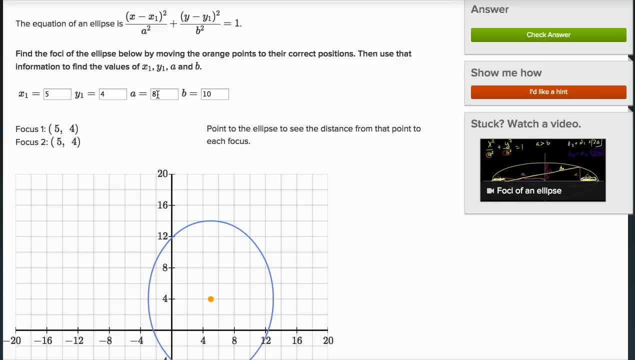 So 100 squared minus eight squared is 100 minus 64, which is 36, and I took the square root of that to get six. 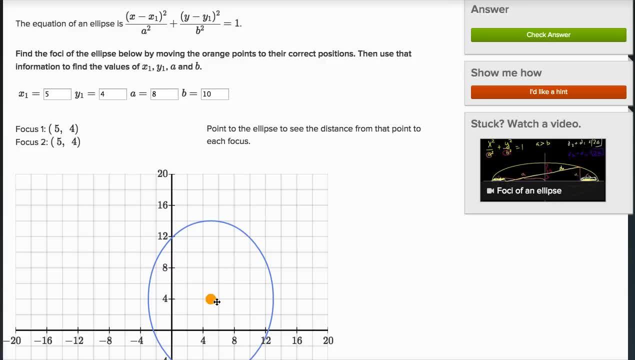 So our focal length along the major axis, I could say, is going to be six. 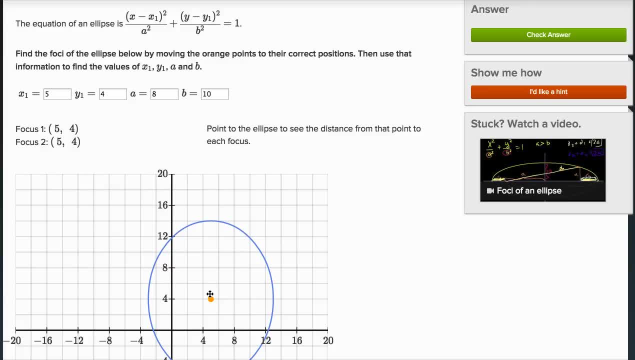 So it's going to be six from the center up and six from the center down. So six from the center up, one, two, three, four, five, six, and six from the center down, one, two, three, four, five, six.